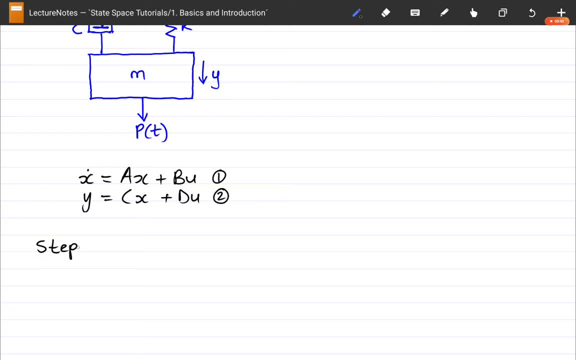 So let's start off with step one. To see step one, we only need to look at the first equation. So let's look at the first part of the first equation, and that's x-dot. x-dot means the first derivative of our state variables. 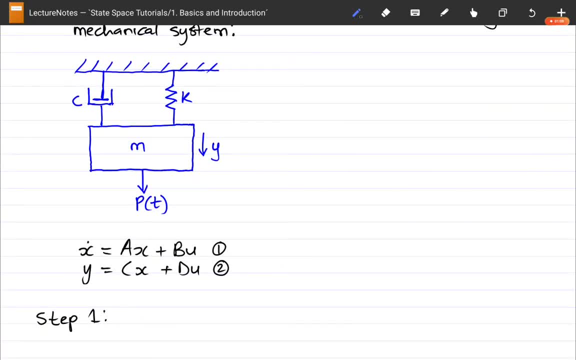 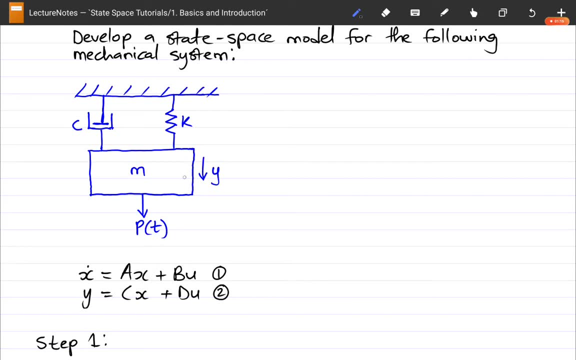 Okay, so that means that tells us that we're going to need differential equations, And fortunately enough, our system here that we're working with has differential equations. We just have to define them or we just have to extract them from the problem for ourselves. 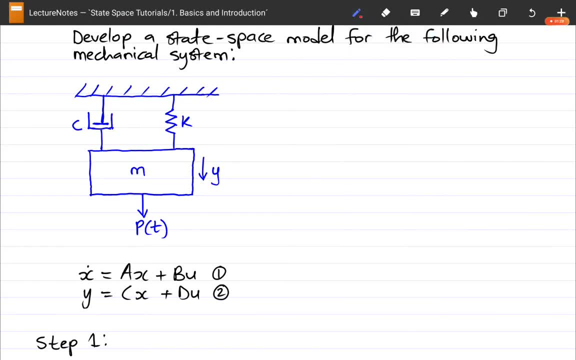 And to do that, we're first going to have to draw a free body diagram, because this is a mechanical system. Okay, so I'm just going to draw a free body diagram here. I should point it out. Free body diagram. This is important. Some can argue that it's not necessary, but I think for students who might find it difficult to solve problems like this on the fly, 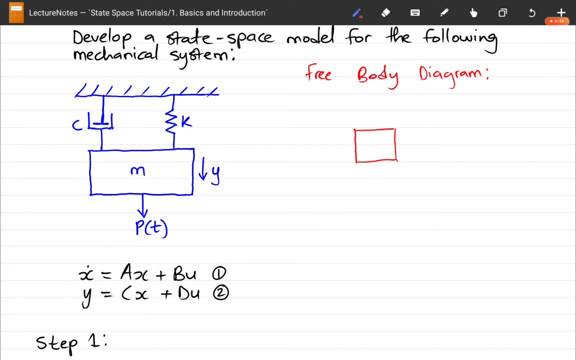 they should start with just drawing the free body diagram. It makes the problem way more simpler to analyze. So all the forces in this system are interacting in the y-direction and that's going to be very important moving forward. Okay, so the first forces acting downward is this p-force, as a function of time, and it's an external force. 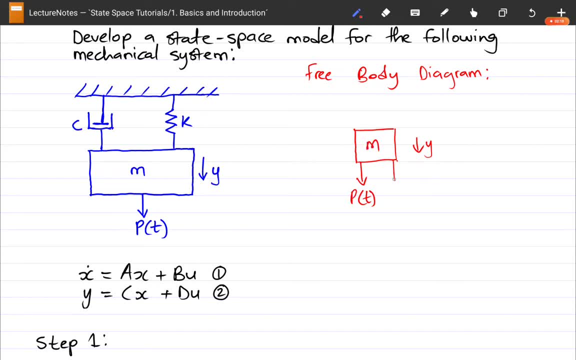 The second force acting downward is the actual mass of the box, which is also acting downward. We can call this force F1.. Okay, And then the forces acting upward are the damper, denoted with C, and the spring, denoted with K. 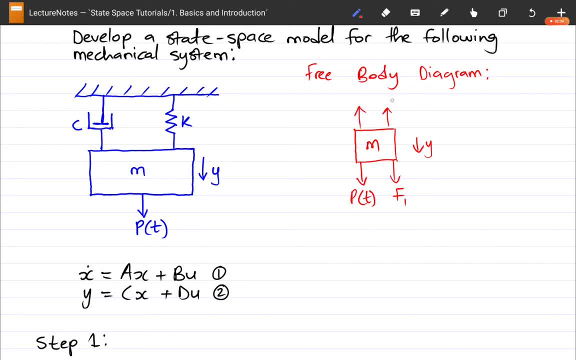 We can show these forces like this And we can say that: C- the force of the damper, is denoted as F1, and the force of the spring is denoted as F3. And this force is F2.. Sorry about that. 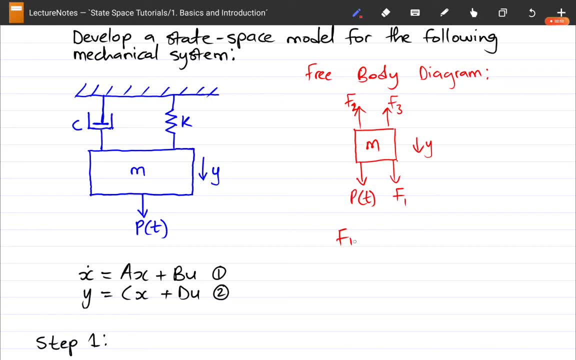 Okay, so now let's define F1.. F1 is the weight of the mass m, So this is simply mass times gravity, and gravity is the second derivative of the direction that this is acting on, The second derivative of displacement, which is y. 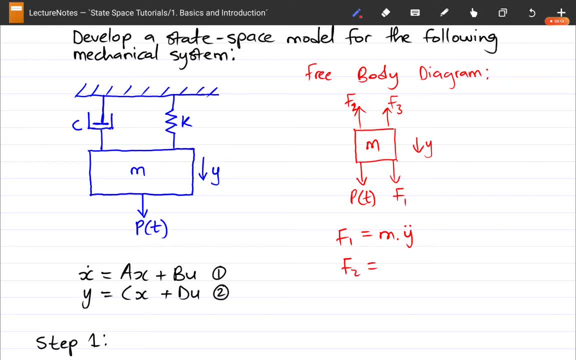 Okay, And then F2 is our damper, which is denoted as C, the first derivative of our displacement. F3 is denoted as the force, according to Hooke's law, as Kx, So here it's going to be Ky. 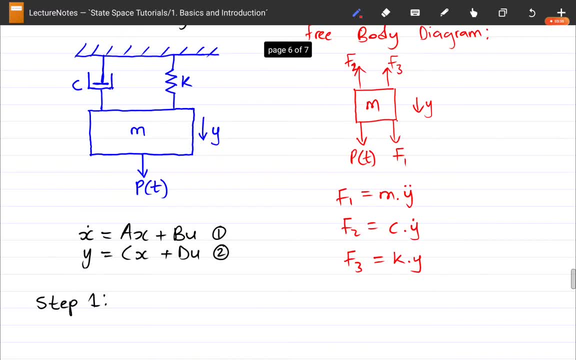 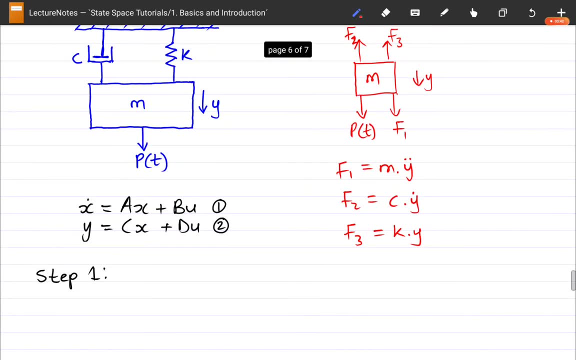 Okay, And Pt is Pt. It is not defined as anything, It's just an external force. Okay, So we've given that. So how can we turn this into a singular differential equation? Well, we can simply say that we assume equilibrium. 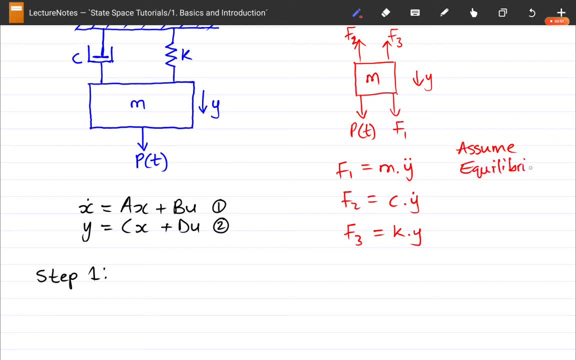 And if we assume equilibrium, then the forces are balanced. The upward forces are balanced with the downward forces. This means that the sum of forces going upward is equal to the sum of the forces of y acting downward, And then that simply means that we can come up with an equation now. 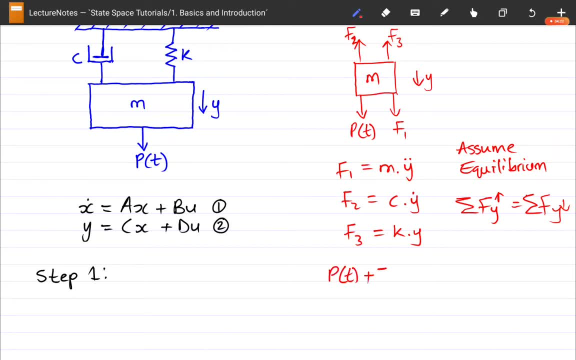 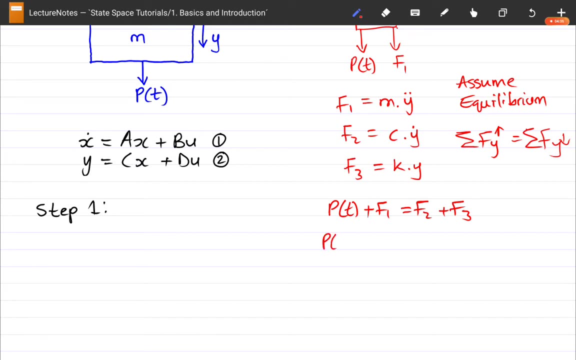 Pt. P of t plus F1. Is equal to F2 plus F3.. Okay, So now we can express this as a differential equation, And then we can write: P of t plus m, second derivative of y, is equal to C, first derivative of y plus Ky. 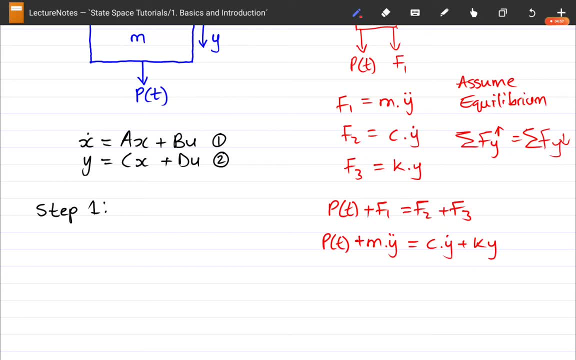 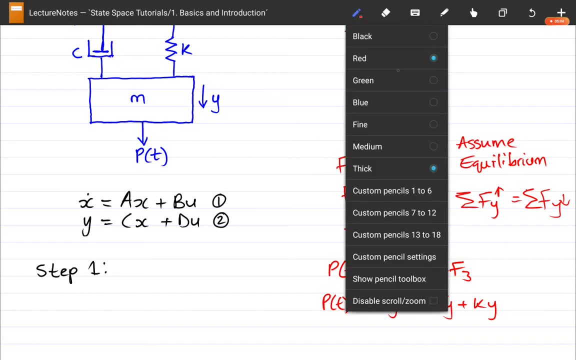 Okay, So now we have our first derivative And then we can work from there. So what do we have to do next? So we can say now, step one is: I'm just going to use a blue pen here. 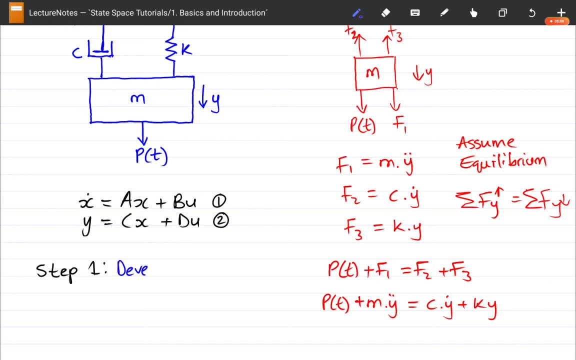 Step one: develop our dE's, And dE's stands for differential equation. Okay, And what would step two be? Let's look at, Let's look again at our system, At our system of equations here. Okay, So we've used this as an idea of how to approach this problem. 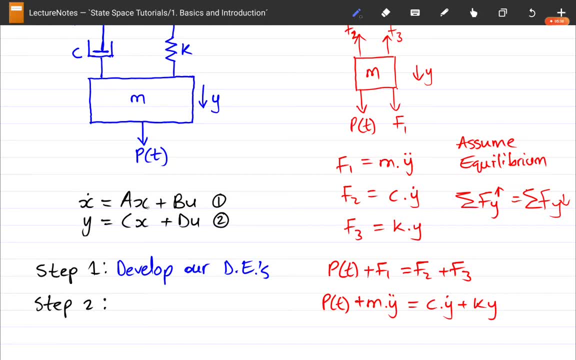 The second thing we need to do is look at, we need to decide on state variables, And that would be for x. Okay, state variables are- How can I describe this? State variables are State variables are State variables are the ones with the derivatives. 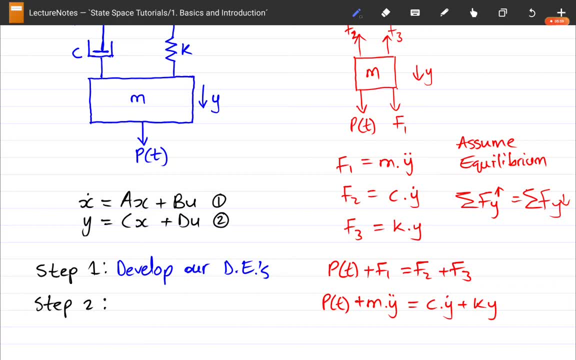 What are being, what is being differentiated here? That's a hint on how we can see them. It's not necessarily the right word, the right way to define it. In the first video, we defined it as the smallest number of a set of variables that can define a system entirely. 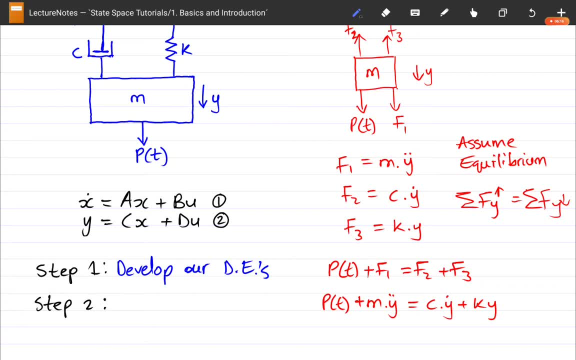 But that example, that definition, doesn't exactly give us an idea here. So here's a hint: State variables are the derivatives. So here, what are our derivatives? Our derivatives are y, That's y, that's being derivated. 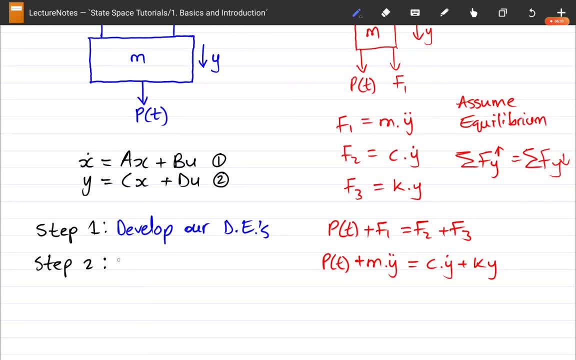 So we can say: step two is identify our derivatives, And I'm going to use a blue pen here. Okay, Identify state variables. Sorry if I'm putting this very close to that And I think I should move that, And I'm just going to try to move this here. 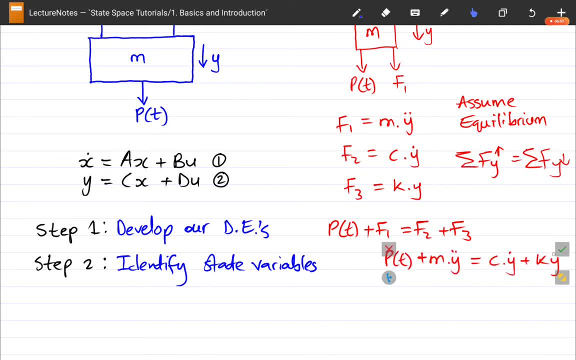 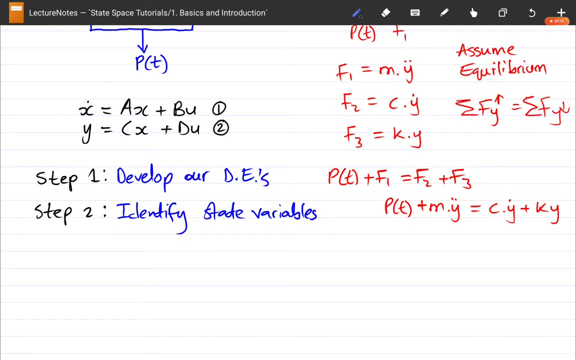 So it can be a bit to that side. Hopefully it doesn't jumble, Okay And then. so now we need to identify our state variables. Okay, So let's say it's y And I want to define my state variables in terms of x here, so that we can be able to have a bit of continuity. 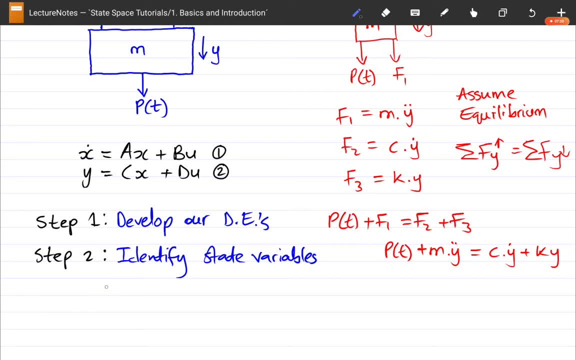 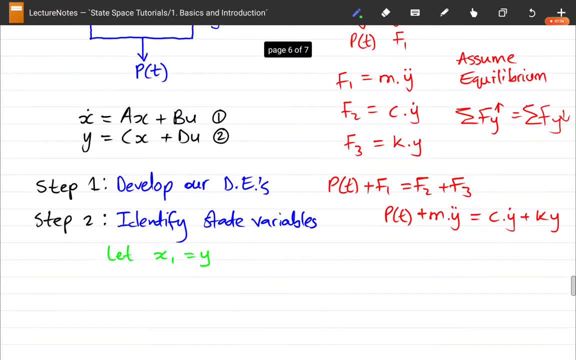 and it's easy to identify what our state variables are, And I will say something like- and I think I will use green here: Let x1 equals to y. That's my first state variable And because we are using y, so that is going to be our first state variable. 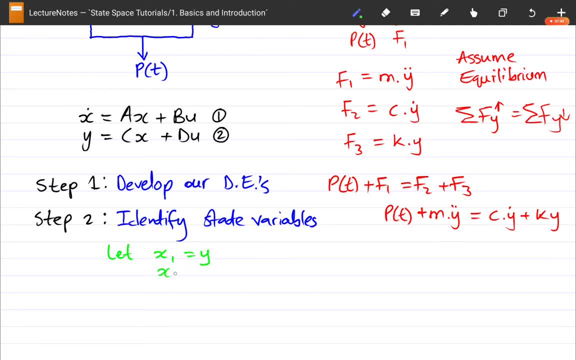 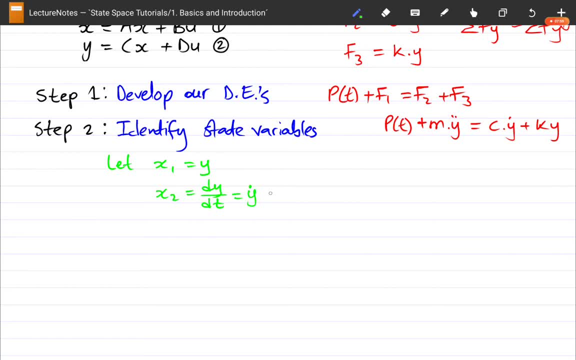 Okay, Notice, this is also equals to x1 dot. That's something worth noting. Okay, So our third one is going to be no. I think that should do it. We should have x2 dot as well. If we're going to have x2 dot, we're going to have x2 dot. 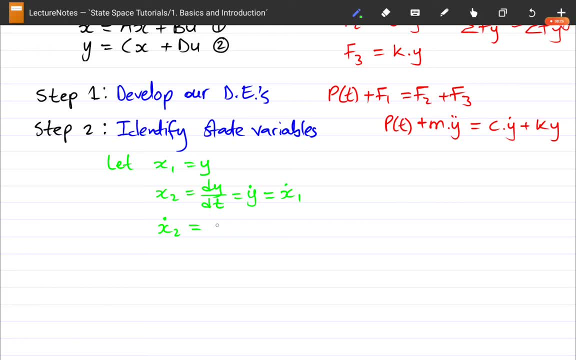 Okay, Okay that, and we're gonna have that x2 dot is going to be d squared, y dt squared, which is going to be equals to y double dot, which is going to be x1 double dot. but we don't have to write that down. 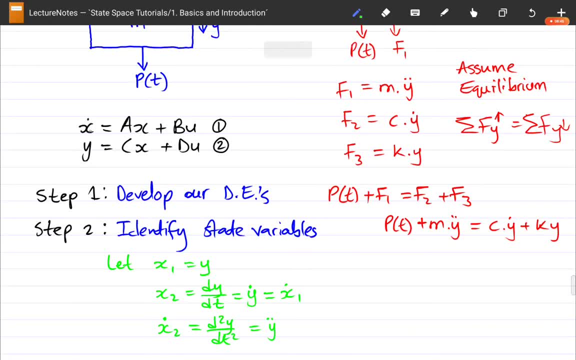 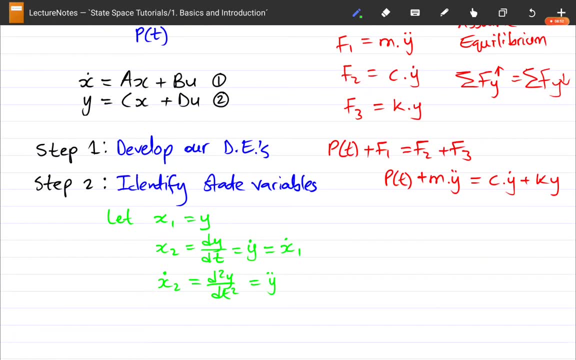 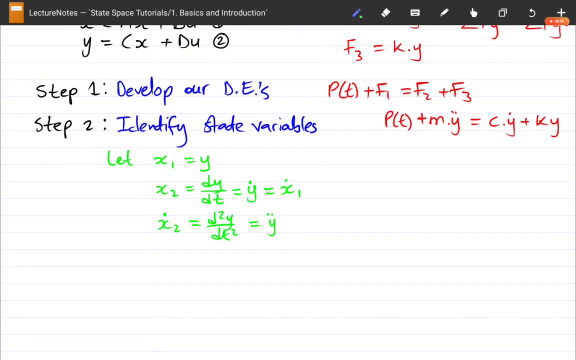 remember for our for x1 dot matrix which we gave here it's only x, it's only one dot, so we don't need two dots on our axis. so now we have this. so what do we do with this? we need to come up with equations for x1 and x2 dot. so look at this: here we already have x1 dot. if I write this in, let me. 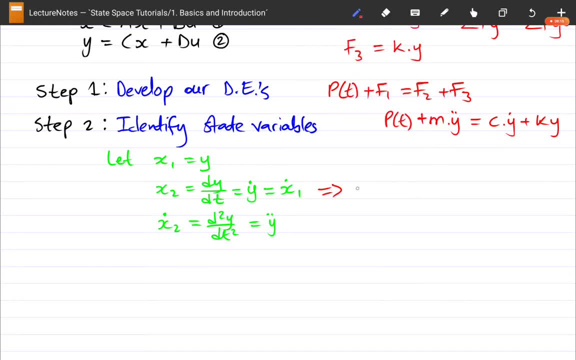 go with red. if I write this in red, we have x1. dot is just equals to x2. okay, but what about this one? can we express this in terms of x1 or x2? no, not directly. so we need to find a way to express this, but we already have an equation waiting for us to express this. okay, 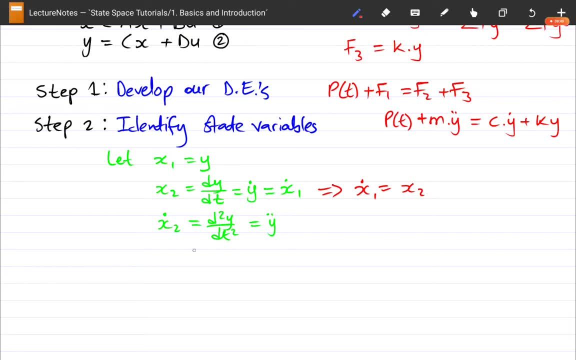 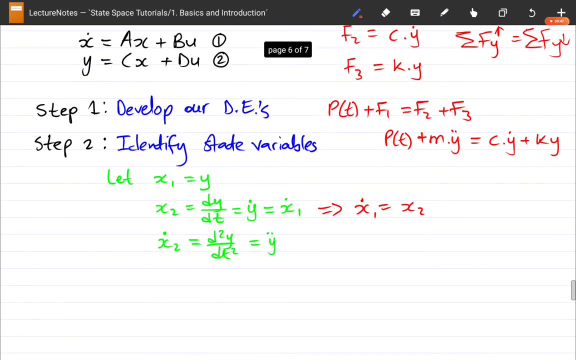 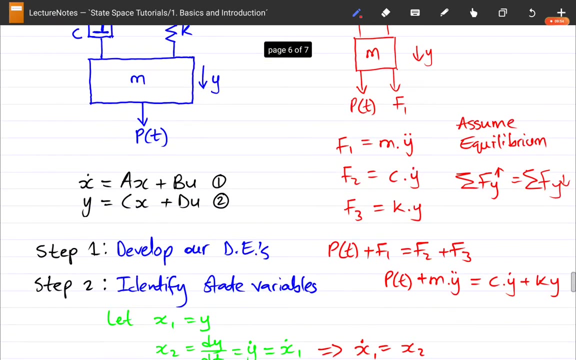 so let's say, we want to remove this P of T, want to express it in terms of something we already have here and what? what we already have here is our vector u and that's our unit vector P. we can write it in terms of the external force, so that's, in a way, an input to the system. so let's, and we 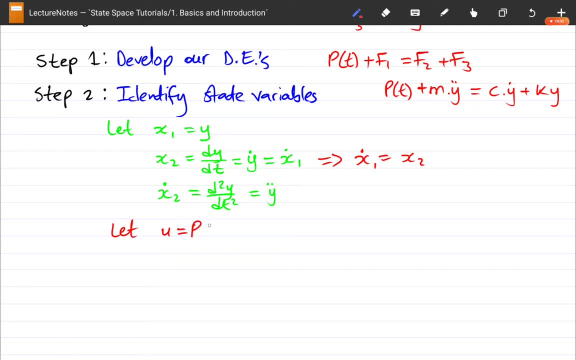 say: let u equals to P of T. that should make life a bit more easier. and now we can rewrite our equation here I can denote it as three. and then we say: three, here is u plus m. and now I give this one as: d squared y, dt squared is equals to C, dy, dt plus k, y. and now we can use this state variables we've. 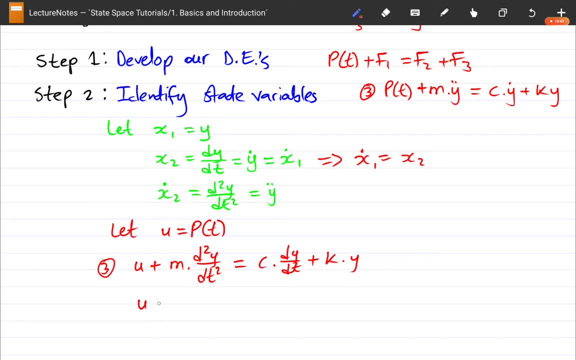 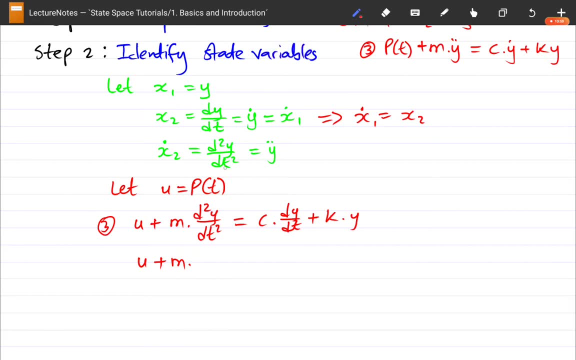 introduced and apply them into this equation, so u stays the same. m obviously is the same and d squared, y dt squared is now our x2 dot, which is going to be equals to C dy dt we discussed. that's our x2 plus k x1. that's a y, y is. 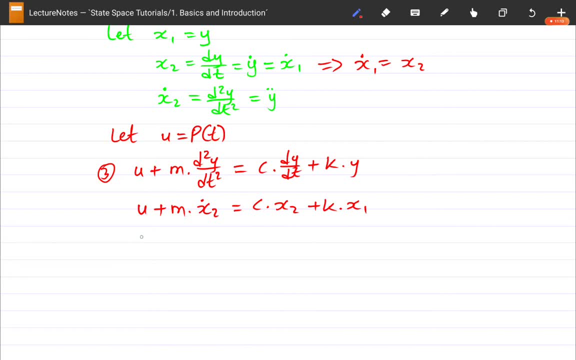 x1. okay, so now we make X dot to the subject. x dot two is equals to. okay, what do we have here? we have c dot, x2 plus k, x1 minus u. that's all multiplied by 1 over m. okay, so this one can extend, so it. 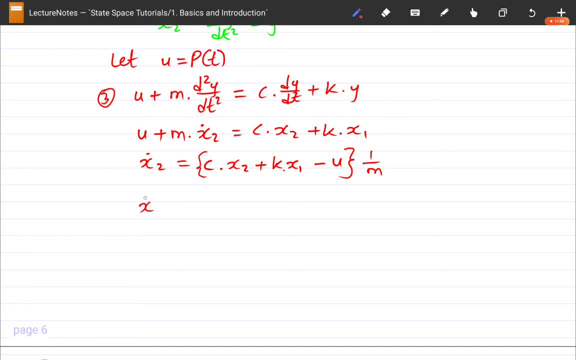 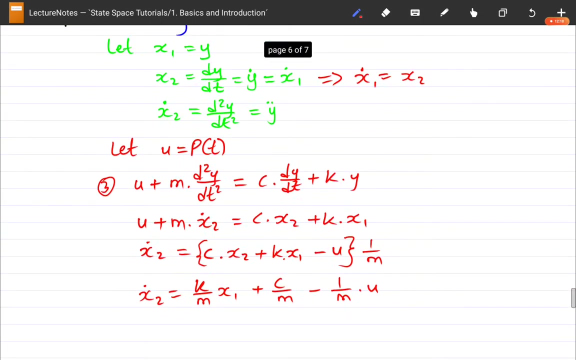 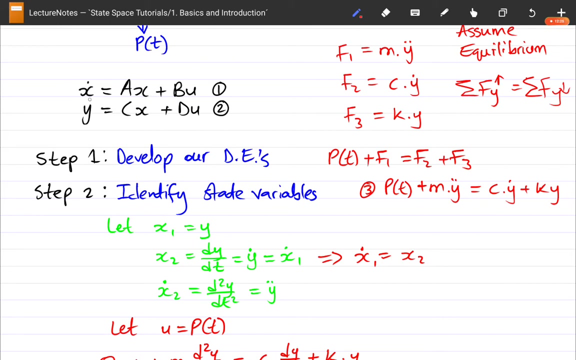 therefore goes without saying that x2 dot is expressed by- and i want to give this in in that order. so i'll say k over m, x1 plus c over m, minus 1 over u, oh sorry, 1 over m multiplied by u. okay, so looking back here, we see we have found our x dot. we have expressed our x dot in terms of: 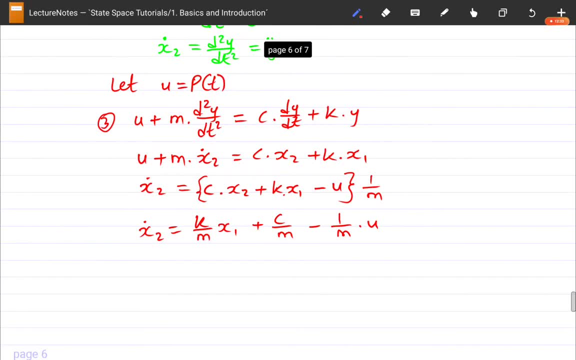 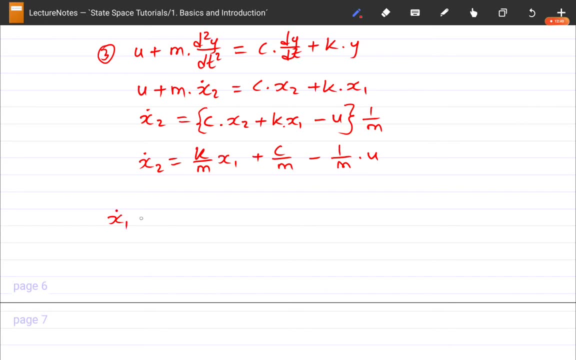 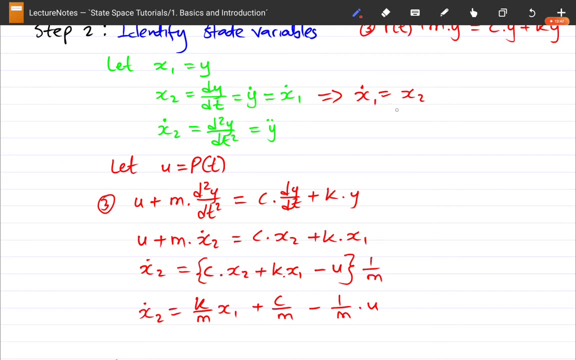 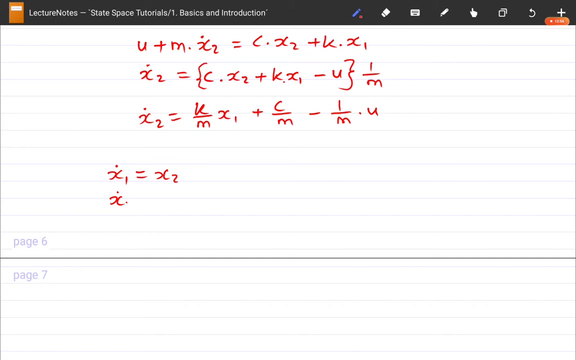 x and u. that's what we've done here. so we can look at it like this: isolating this, we can say: x1 dot is equals to: and if you look at it here, we did discuss that x1 dot is equals to x2 and x2 dot. we just copy this one here. that will think I. 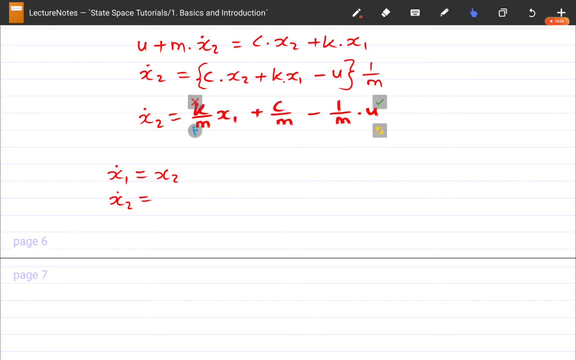 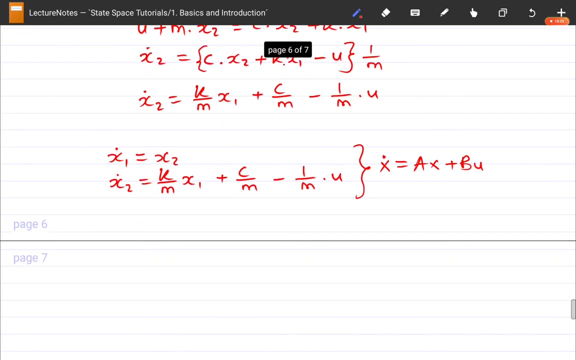 will literally just copy that there and we put it here, and then we have our, our first equation. it's not obvious, but this looks exactly like: x dot is equals to a X plus B you, and we're going to write it in matrix form. not so long and not so. 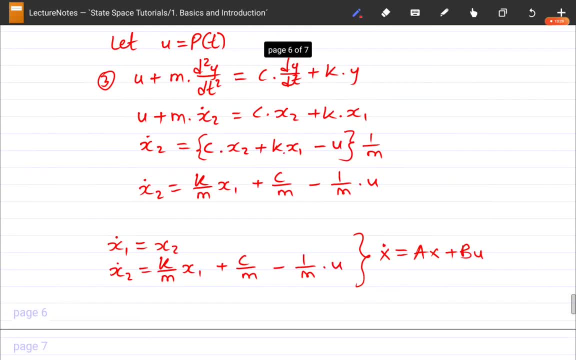 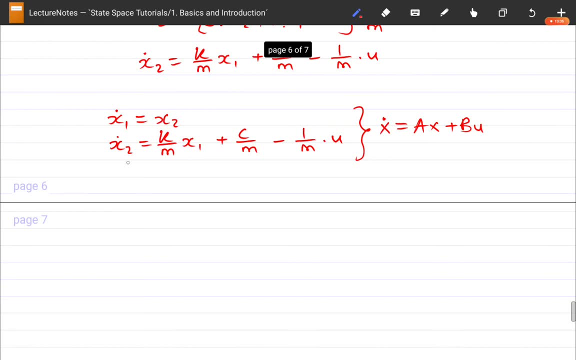 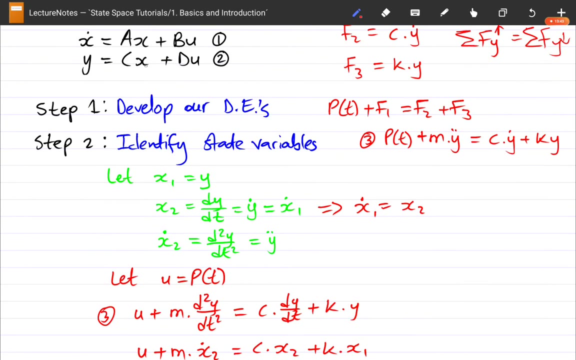 long from now. and then we have our other one, which must be expressed in terms of y, which is: y equals to C, X plus D, u. okay, so y has to be expressed in terms of y, X and u. so let's find, let's see if there's a relationship somewhere here. 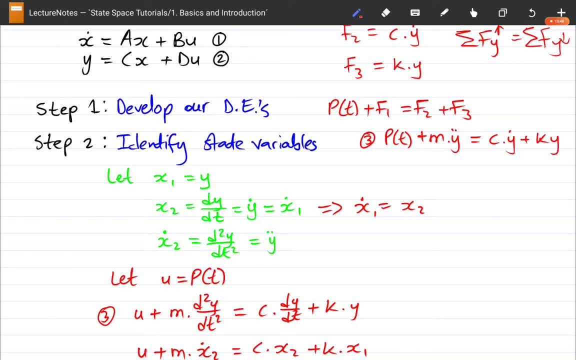 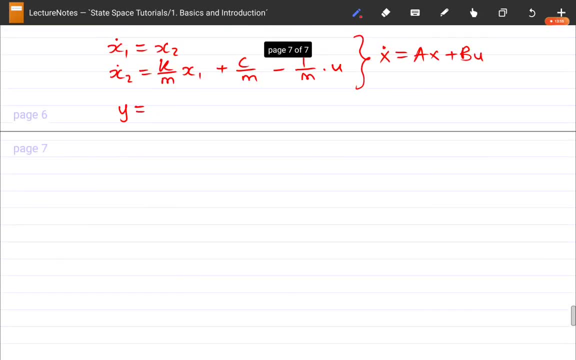 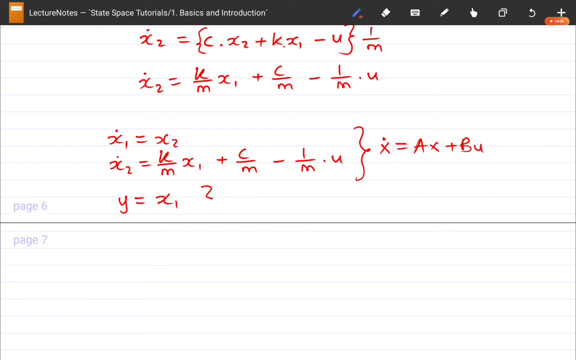 that at least expresses y in terms of any of the state variables. and looking immediately, we can see here y is just equals to x1. so we already have an expression for that. so y is equals to x1 and this is our y is. it was to C, X plus. 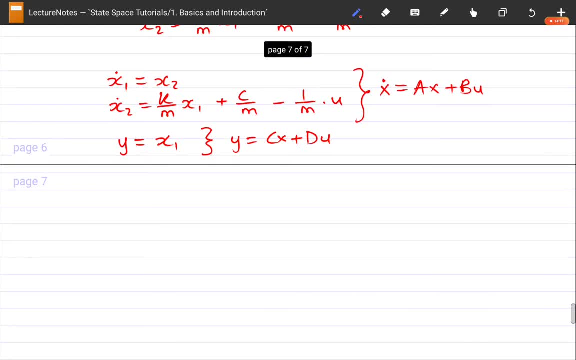 D? u. so we should be able to write this in matrix form so we can see now X 1 dot next to dot. it was to okay, so x 1 x 2 x 1 is just close to next to. so if I wanted to multiply this, 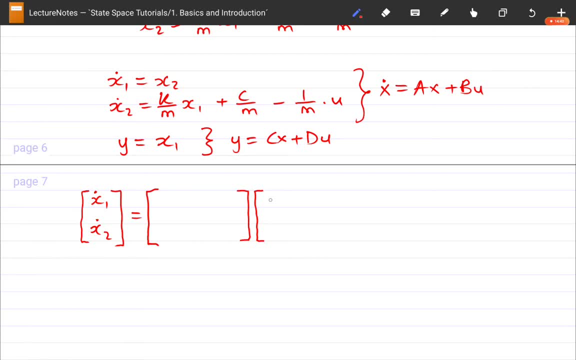 with X 1, so we say x 1, this one's going to give us x 1, that's going to be x 2. This is this only has an x 2 component, Which is much, which is a coefficient of 1, and it doesn't have anything with a coefficient of x 1. it has a x 2 core. 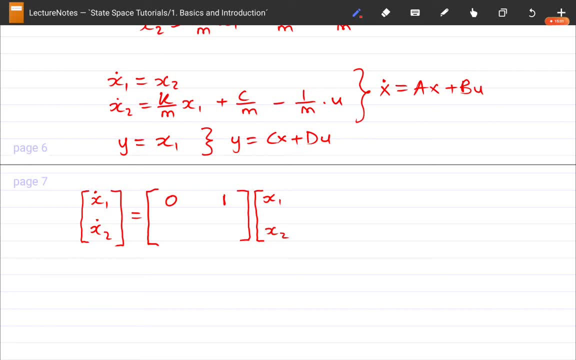 Coefficient. that's why. so I hope everyone remembers their linear algebra. Okay, so the next one is x 2, dot x 2, that is K over M. That's the coefficient of x 1. Okay, and then the coefficient of X, or sorry? 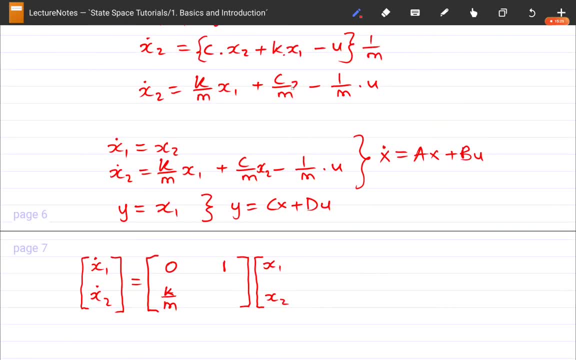 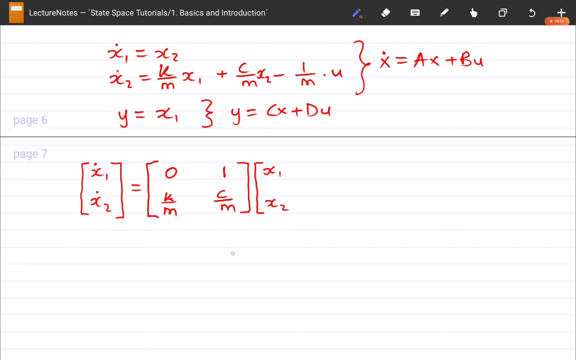 That was supposed to be. the wonder why that wasn't there. I Mistake. okay, so that's going to be C over M And we can close that now, and then we're going to have our coefficient of u, Which is going to be minus 1 over M. 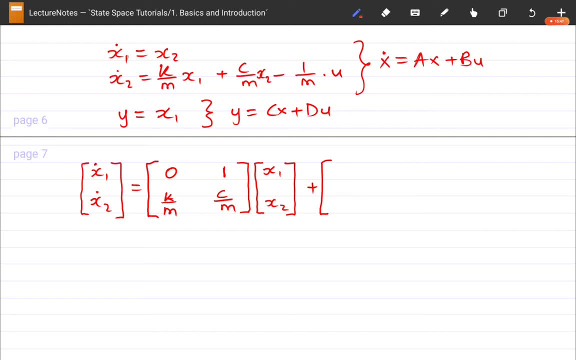 And this only applies for x 2, for 0, for X dot 1, which is this one, it there is no relationship of you, so it is not working in terms. It doesn't. it doesn't require the input X dot 1. That's what does the observation we can make from that? okay, and then we have this one as 1 over M and 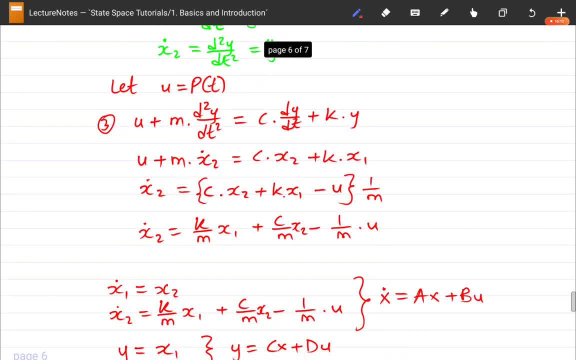 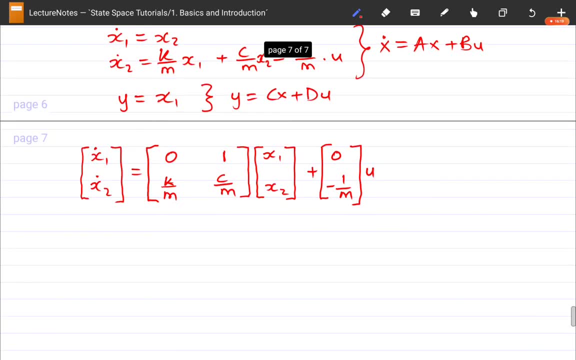 Because we don't know what the value of u, which is p of t, is. we just leave it as a matrix like this. You or you can give it as p of t, okay, and then why? because it's a function of, it's just a. 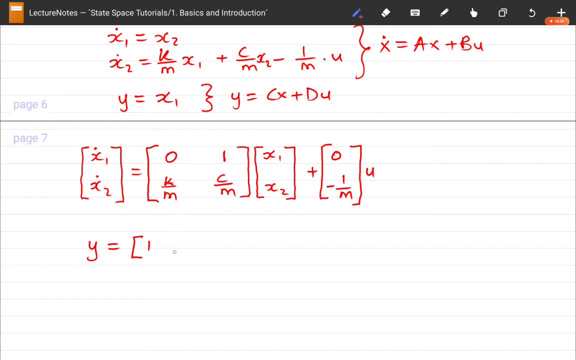 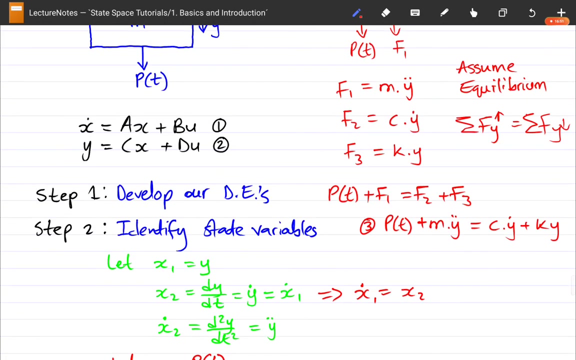 Function of x 1, then we can just say it's 1: 0, X 1 and x 2, Which literally means the same thing as y is was to x 1 and just like that We have expressed our state space model By using all that, just by following these steps. 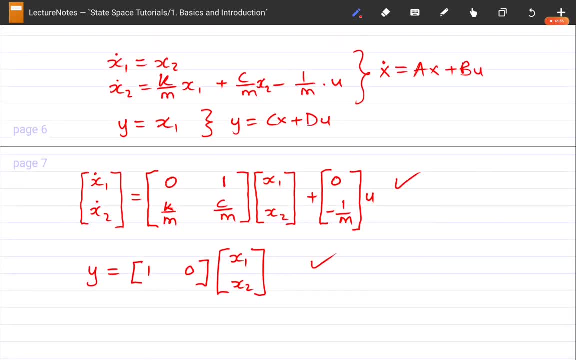 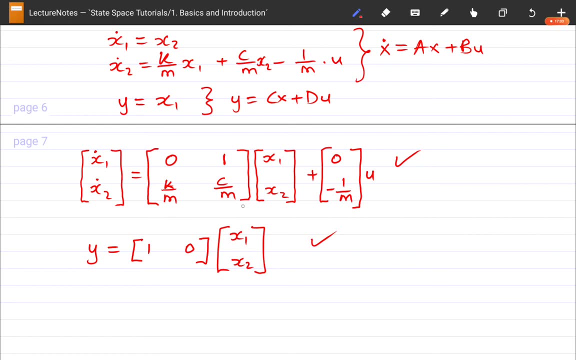 Okay, I hope that made a lot of sense. and so what can we take from this? What does this tell us about our system? Remember, we said that this vector, this matrix here is called our system matrix and, as you can see, it has all the parameters of our